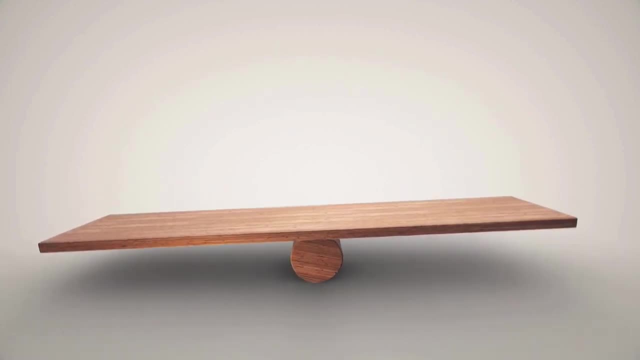 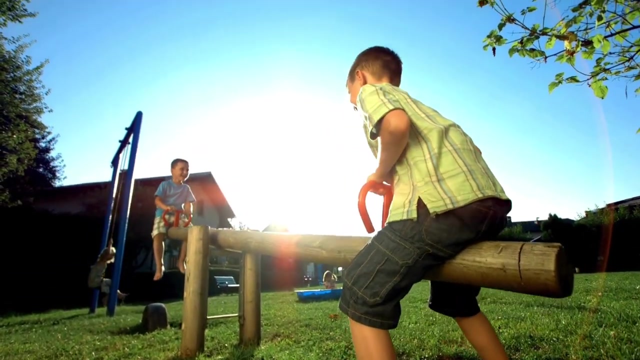 If you know what a seesaw is, then you know that pushing down on one side is applying force, And this is what makes the other side go up, lifting you into the air. And this is what makes the other side go up, lifting you into the air. 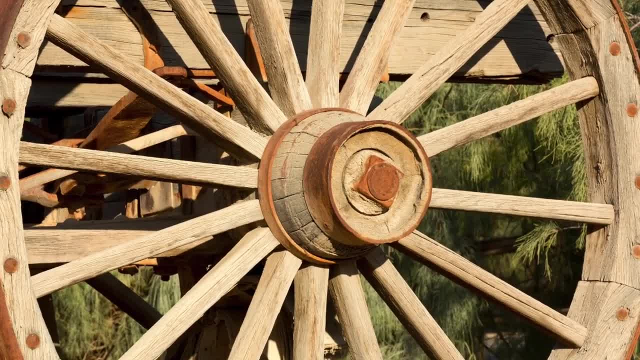 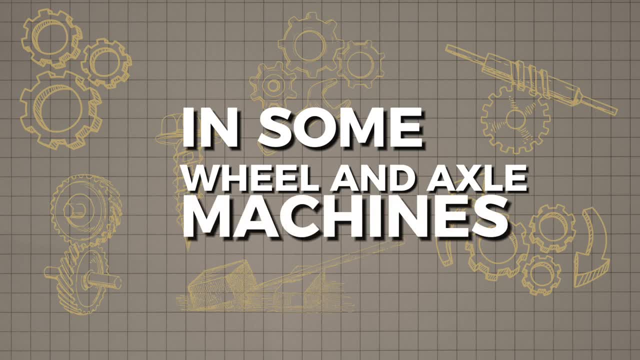 Next we have the wheel and axle. An axle is a shaft or rod that is fixed to the center of a wheel. In some wheel and axle machines the wheel is replaced with a crank or another part that spins in a circle, just like a wheel. 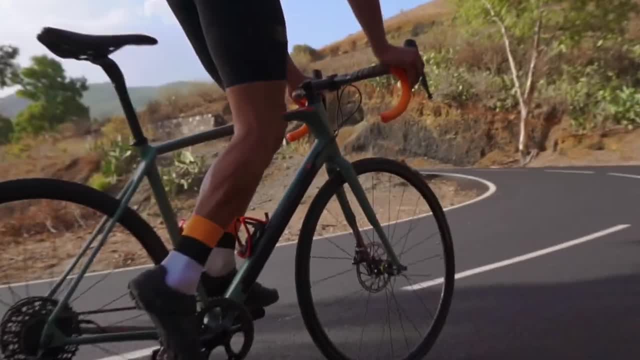 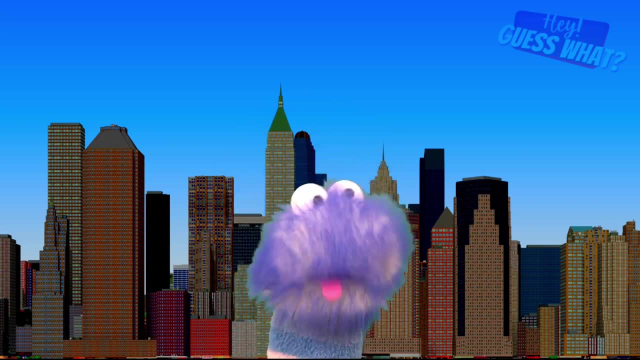 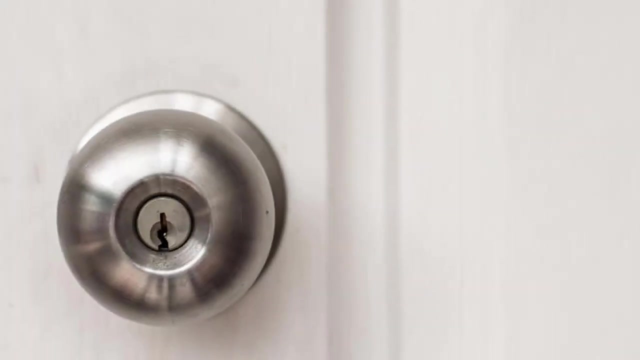 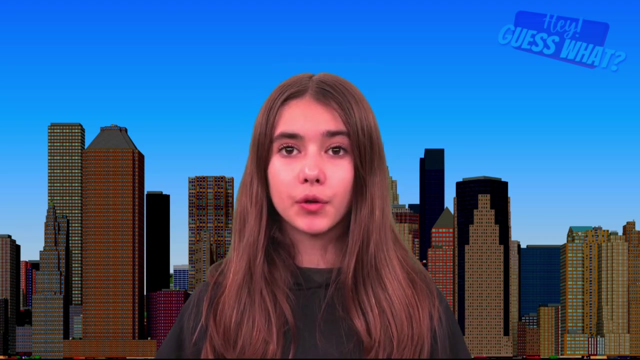 Wheels help things move smoothly, like on a bike or a car. The wheel and axle help you move things easily by rotating. A steering wheel in a car is a wheel and axle machine. Another example is a door knob. A door knob is a wheel that turns the inner shaft or axle. This is what moves the latch. 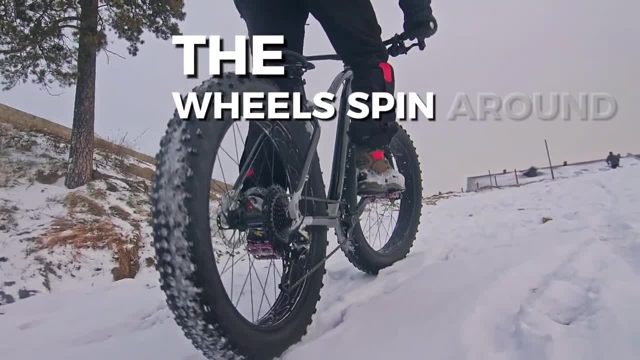 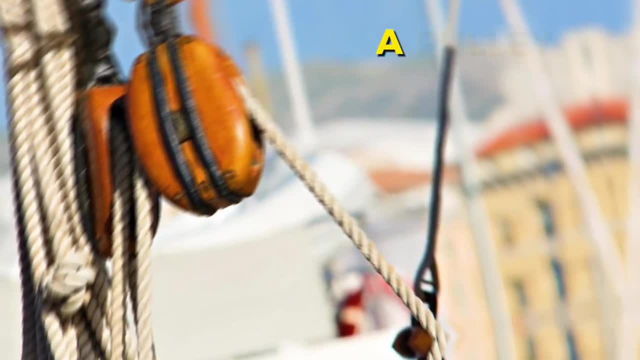 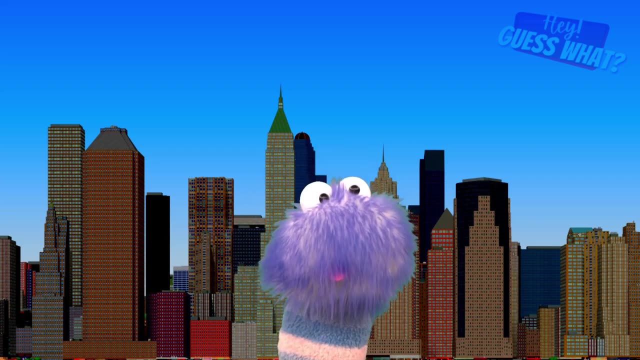 On a bicycle, when you pedal, the wheels spin around the axles, helping you move forward smoothly. Next we have a pulley. A pulley helps you lift stuff up much easier, even heavy things that you couldn't pick up with just your hands and muscles. 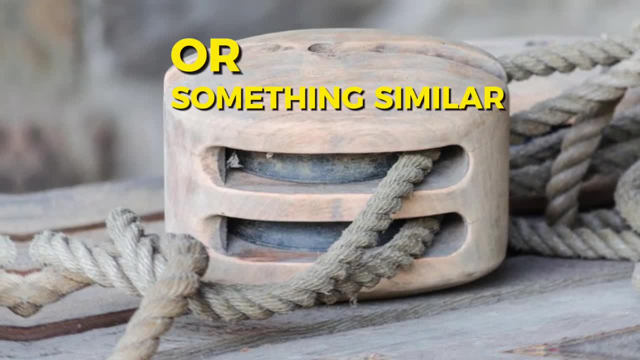 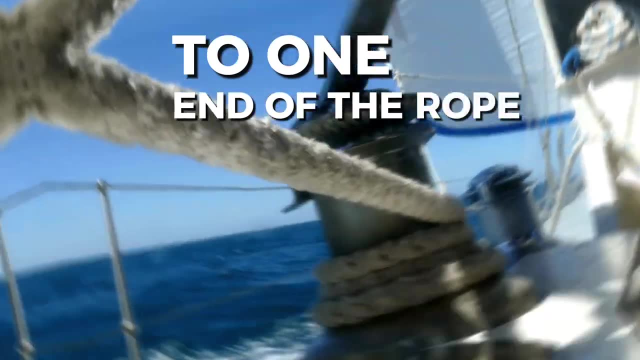 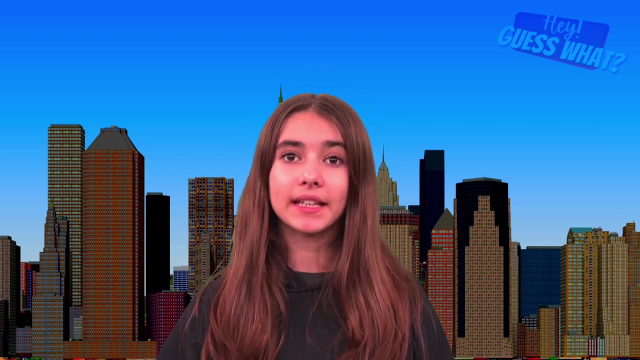 A pulley is a wheel with a rope or something similar. around its edge, The pulley changes the direction of the force applied to one end of the rope. Think of raising a flag on a flagpole. Pulling the rope makes the flag go up without needing to climb the pole. 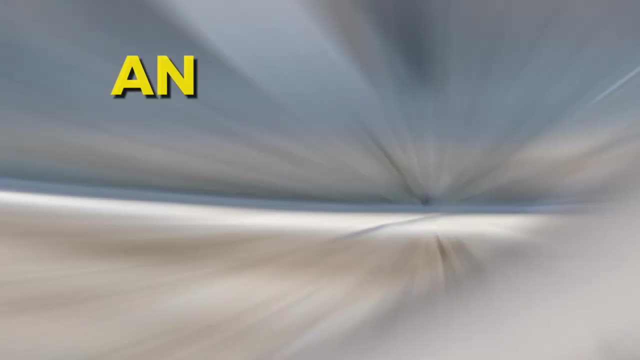 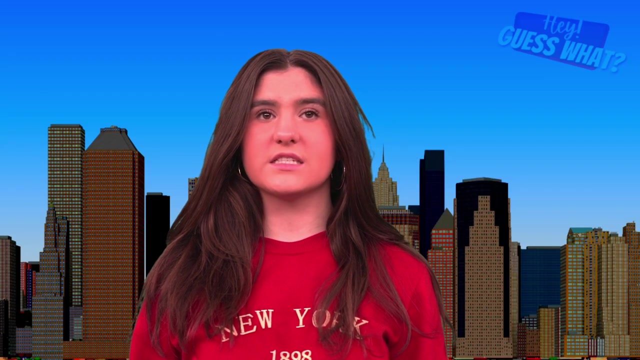 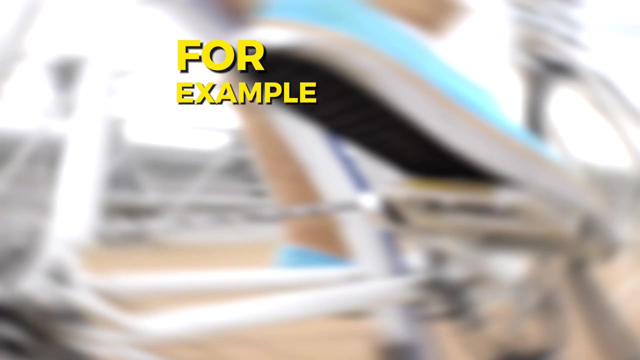 Next we have an inclined plane. An inclined plane is a flat surface with one end higher than the other. Inclined planes are like slopes that help you move things up or down with less effort than lifting straight up. For example, riding your bike up a ramp is like using an inclined plane. 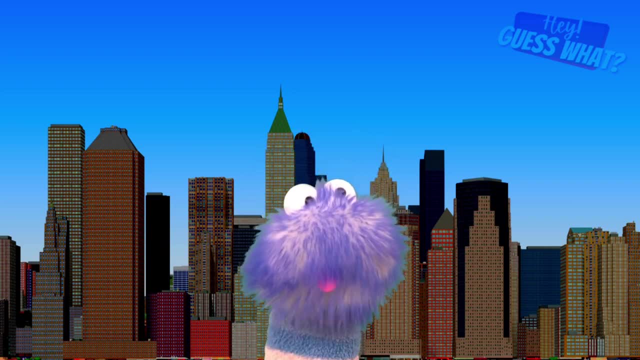 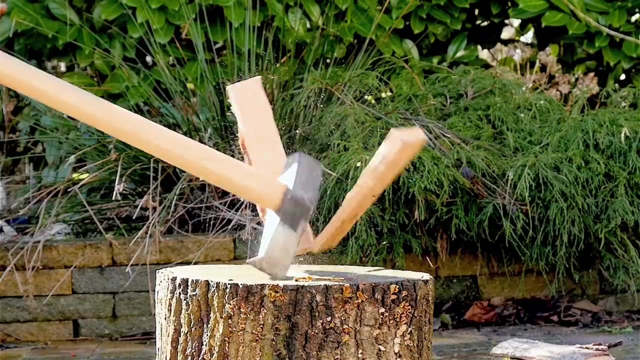 The next simple machine on the list is a wedge. A wedge is a piece of material that narrows to a thin edge. Pushing the wedge in one direction creates a force in a sideways direction. The head of an axe is a wedge. Swinging the axe into a log can split the log apart.